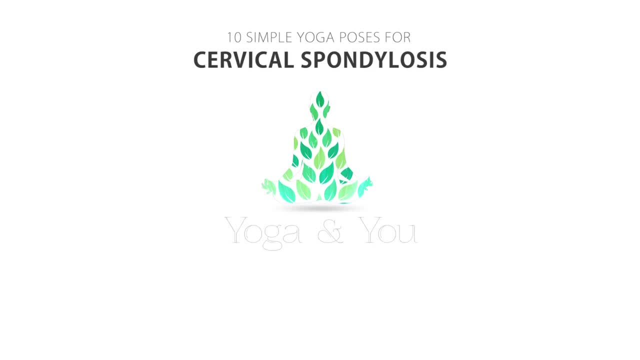 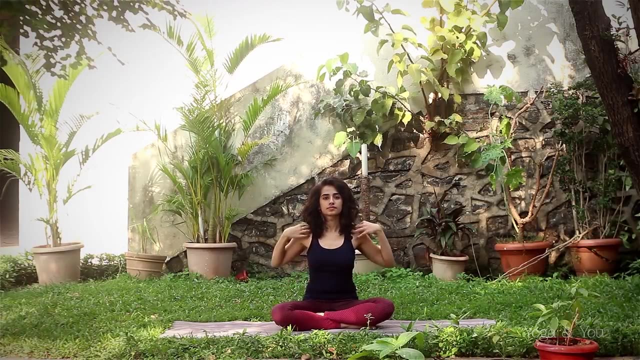 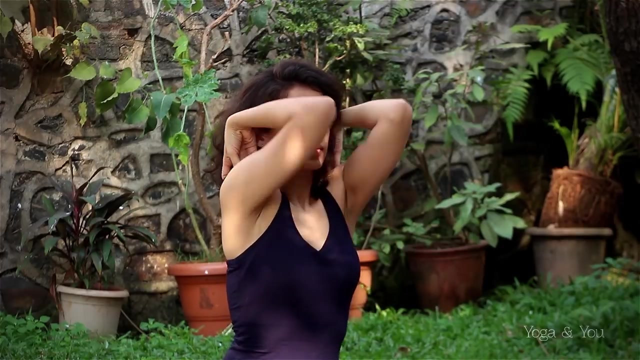 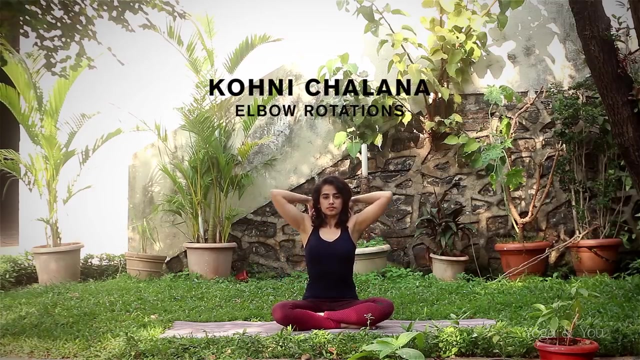 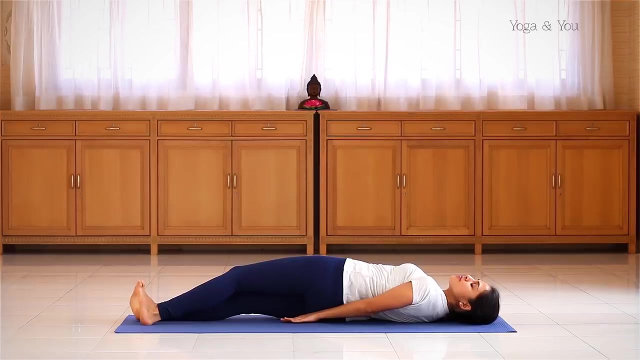 As we start with shoulder circulation, clockwise, trying to meet the elbow in the center and reversing anti-clockwise From the supine position. place your palms down and bring your hands underneath the body with the elbows as close to each other as possible, Feet together, Inhale. 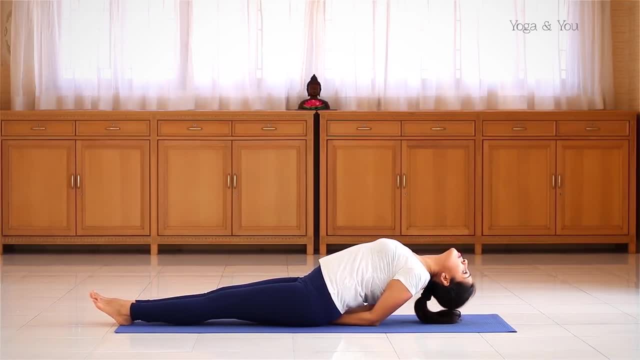 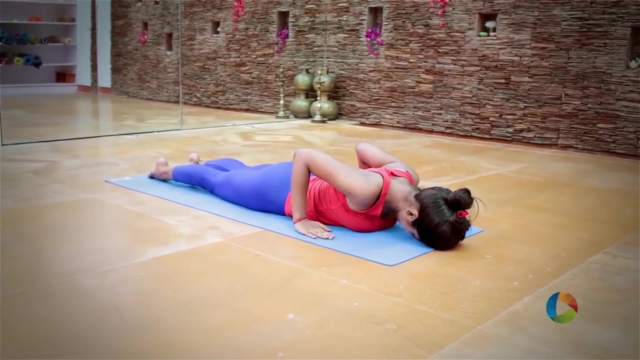 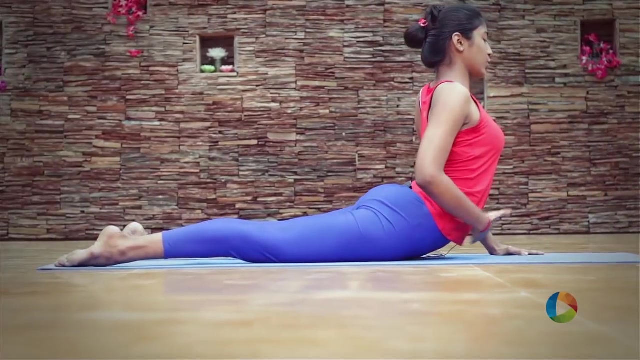 lift the head up. Look at your feet, Exhale. bring the crown of your head onto the mat. Open the shoulders Now gently place your hands down in between your shoulders and your pelvic bone. Open your legs slightly out, Inhale and then come up. Now lift your navel above the ground. 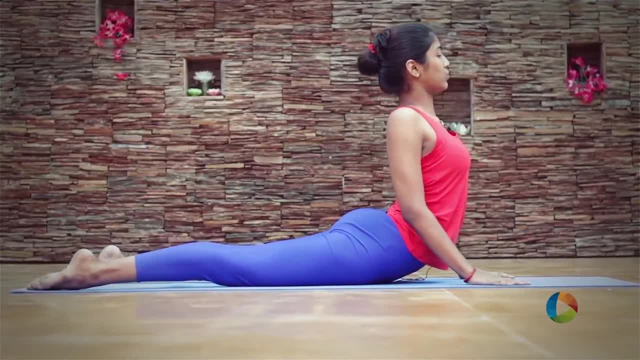 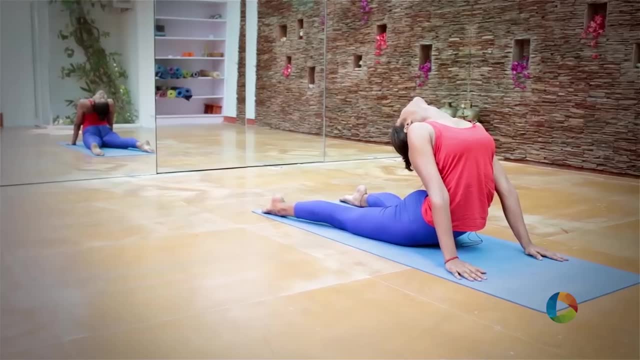 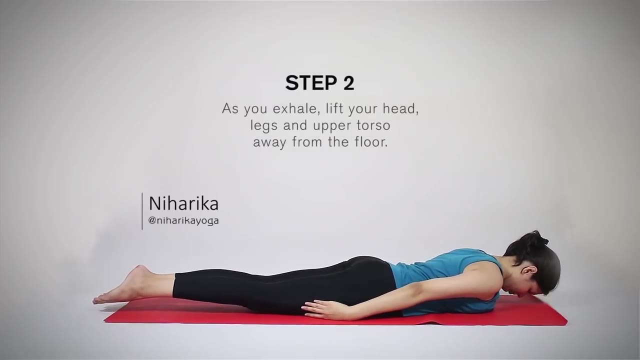 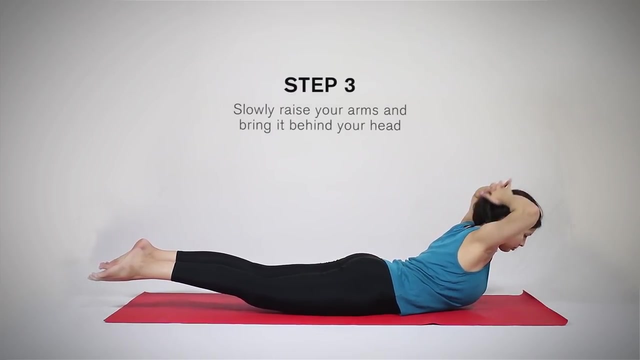 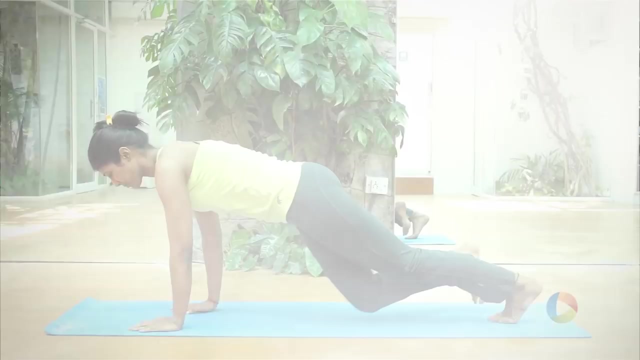 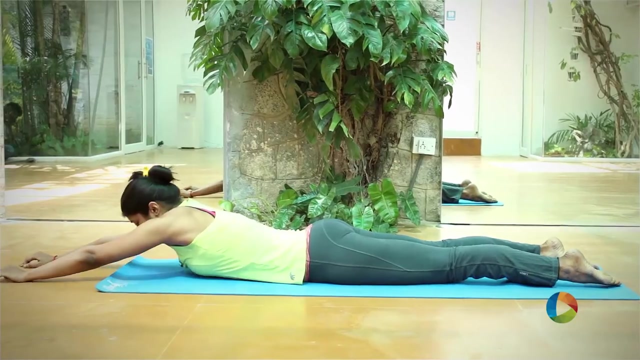 level. Push your pelvic bone down. Procure your pelvic bone down and then elbows straight, Push the shoulders back. Stretch your hands forward, Your legs out, Lengthen your spine. Feel someone is pulling your hands forward and then your leg back. Stretch your hands back, Pull your legs up, Inhale, lift your hip. Inhale. lift the head up and inhale. Exhale. pull the lower leg up and exhale. Tilt your hands in the front and exhale Three more times. This time you can feel the relaxation in your core muscles and 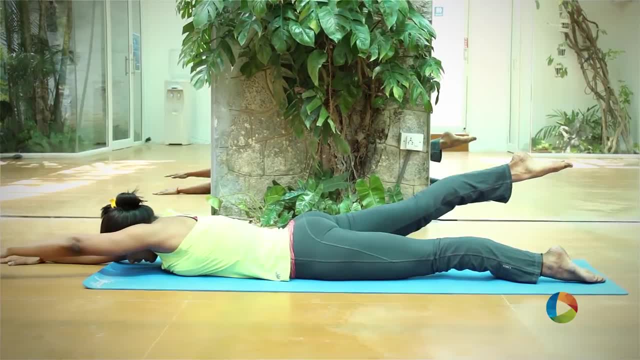 your foot. This is a very different exercise for the outer thigh muscles and this exercise can be done nicely. now inhale, lift your right leg up and then your left hand up. gently lift your head up, look at your finger points, or else you can look at the ceiling. stay. 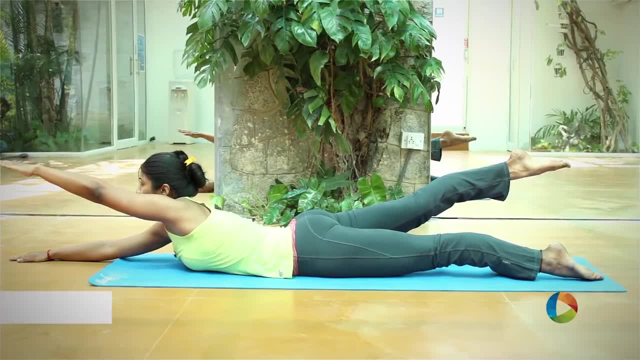 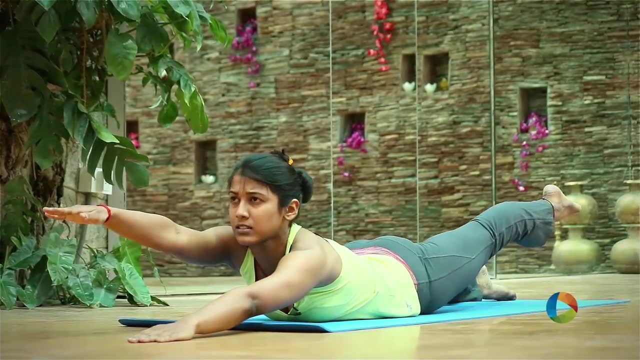 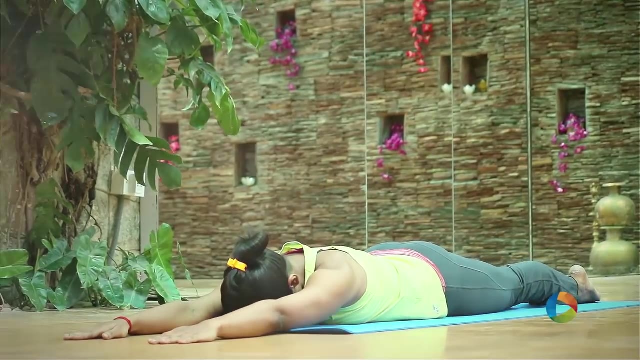 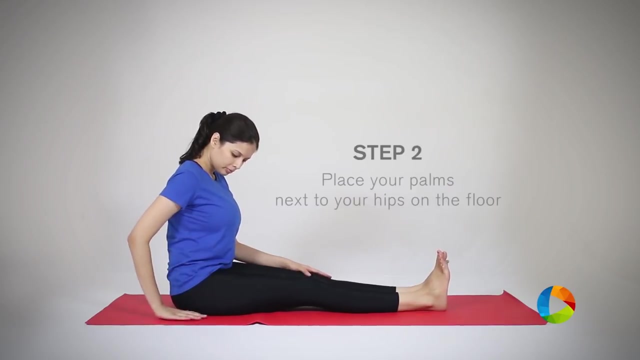 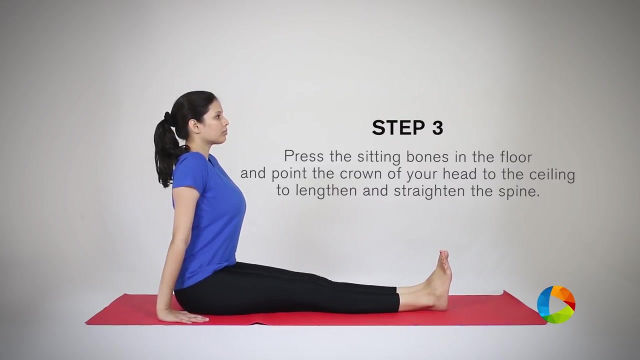 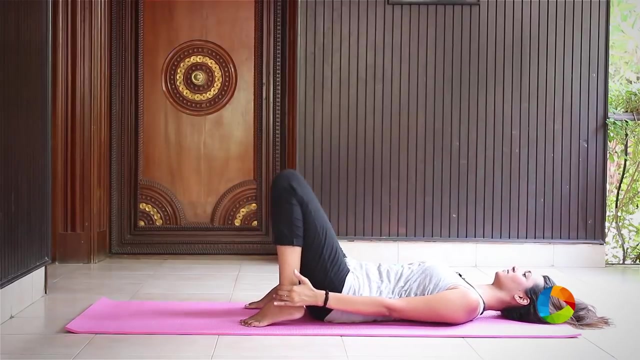 here for five to six breaths. exhale down again. repeat it with your other side, point your toes, exhale down and begin to lie down on your back. begin to lie down on your back and place your heels as close as possible to your butt and hold your ankles. make sure your thumb is outside and. 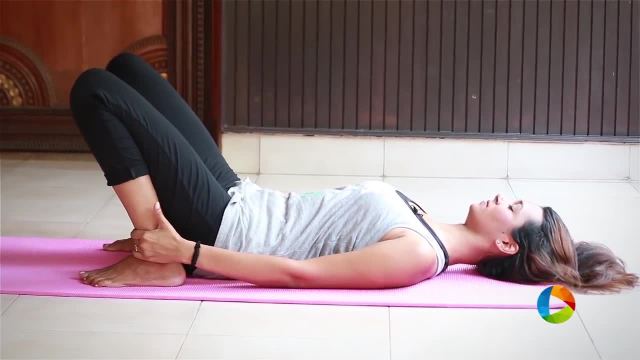 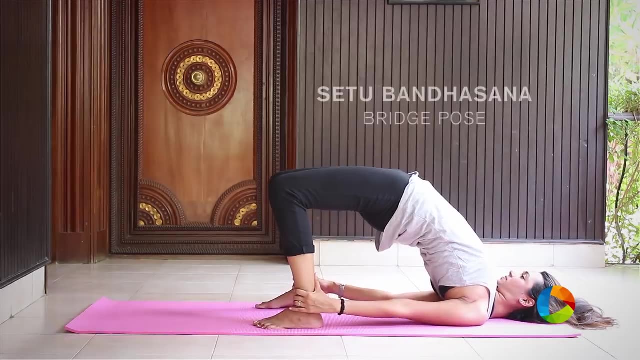 hold your heels, make sure your thumb is outside and, When you're ready, slowly inhale and lift your hips all the way up. So try and reach as high as possible, but your breath should be in the normal range and Stay here for a couple of deep breaths. 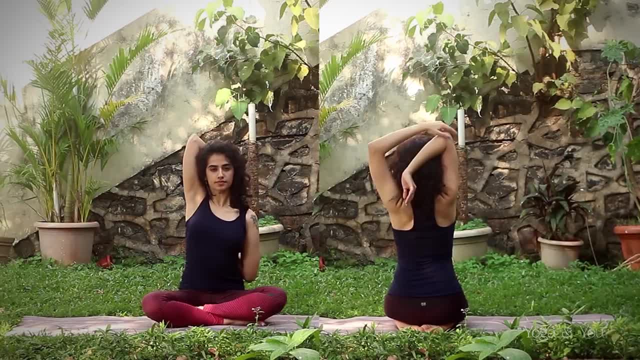 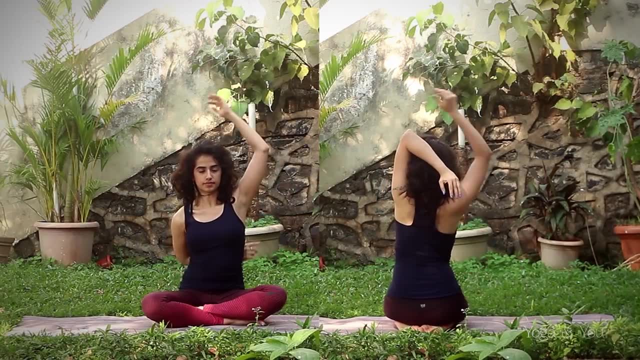 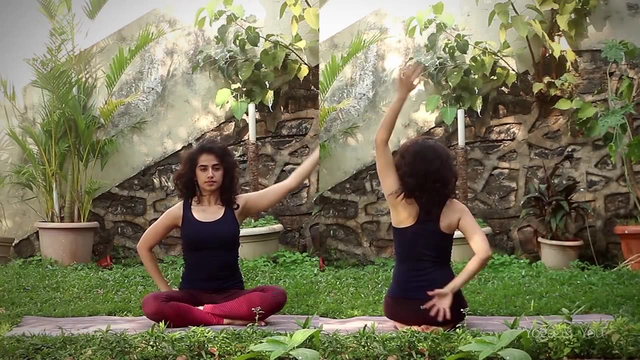 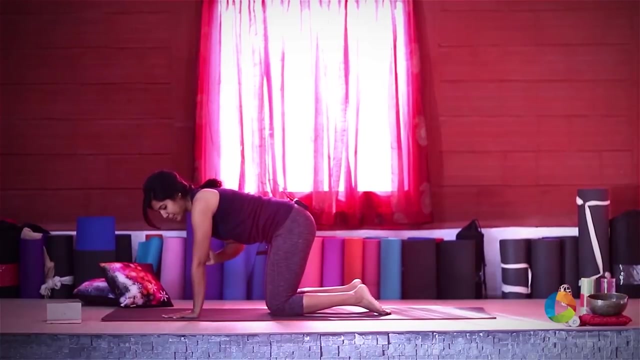 Next, moving on to Gomukhasana hands, starting with the right hand meeting the fingers behind the back. If your hands cannot meet, you can use a belt or a hand towel. Come into all fours. So what that means is you need to have your wrists Always aligned underneath your shoulders and your knees always aligned under the hips. 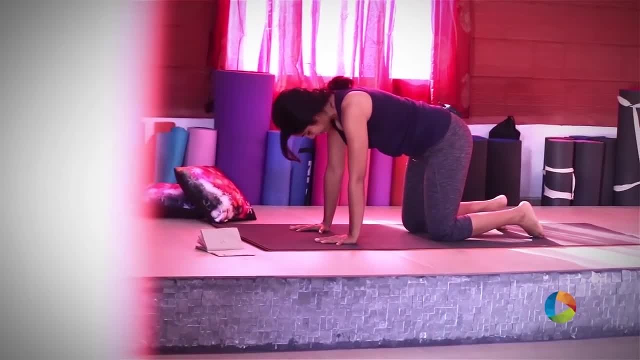 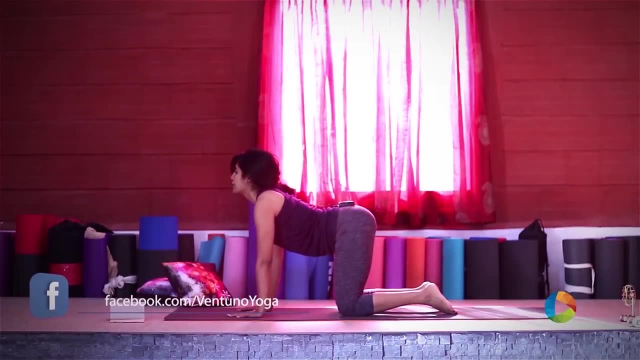 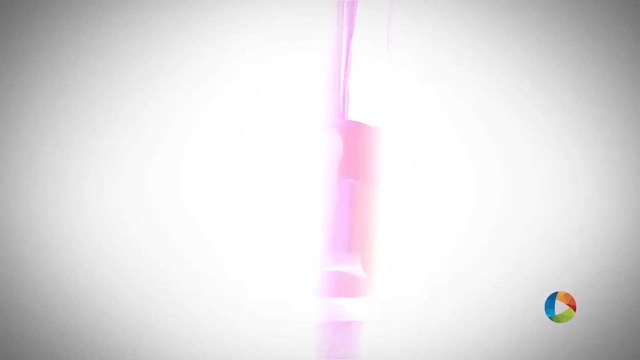 Your hands are shoulder-width distance and your knees are hip-width distance. What we are going to do is drop the spine down as you lengthen upwards, with the chin and the tailbone On the exhale, you'll round through the shoulders, pull the belly in and bring your chin to your chest. 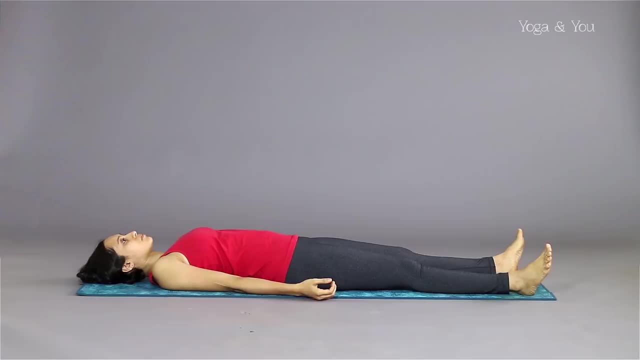 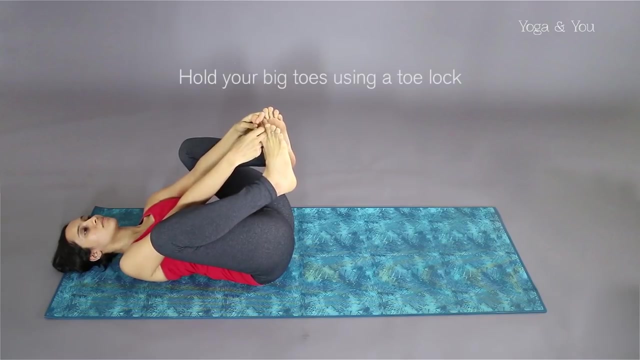 As you look to your navel, come to a neutral spine, lie flat on your back, Inhale and slowly bring your knees close to your chest, With the arms stretched on the inside of the legs. hold your big toes using a toe lock and Gently open up your hips and legs. 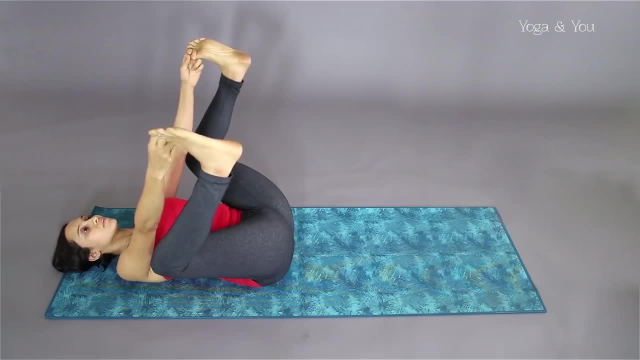 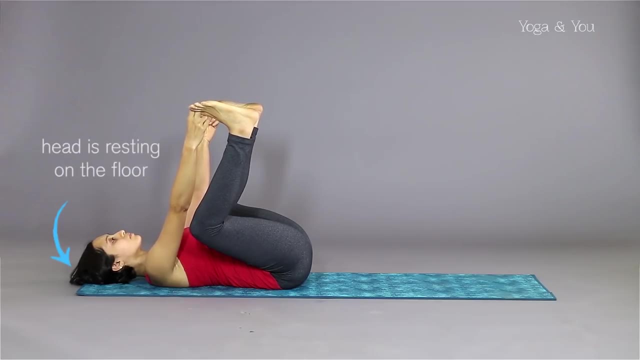 And widen your legs to deepen the stretch. Please make sure your head is resting on the floor. Stack each ankle directly over the knee so that the shins are perpendicular to the floor. Press your tailbone Sacrum down to the floor while you press your heels up, pulling back with your arms.